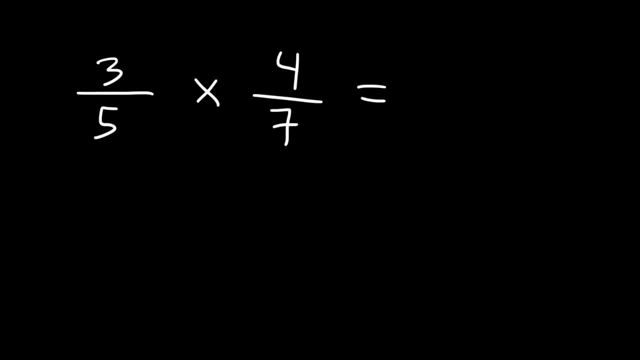 See if you can get the answer. So what do we need to do in this problem? How can we multiply these two fractions? When multiplying fractions, you need to multiply across. So we're going to multiply 3 and 4 together. 3 times 4 is 12.. 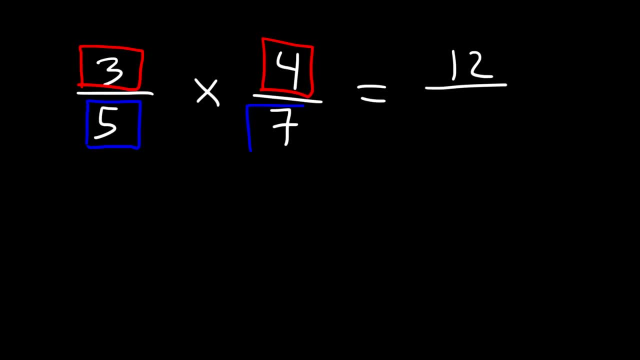 Next, we need to multiply the two denominators together. 5 times 7 is 35.. And so that's it for this problem. That's all we need to do, And the answer is 12 over 35.. Now it's important to check and see if you can reduce the fraction. 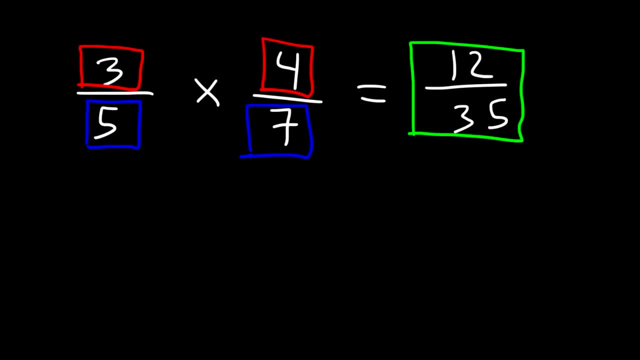 And for this example we can't simplify the fraction, So the final answer is 12 over 35.. Now let's try another example. Go ahead and multiply these two fractions: 2 over 5 times 3 over 11.. 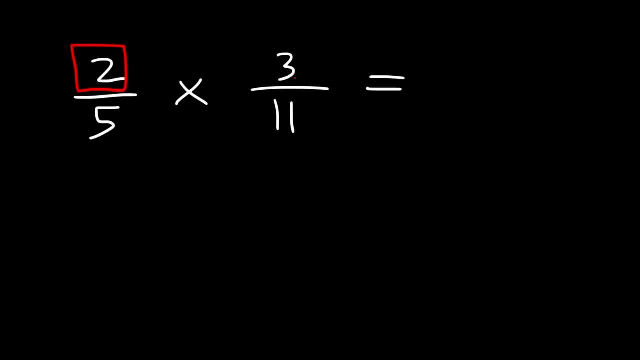 So once again, we're going to multiply across: 2 times 3 is 6.. And then we're going to multiply 5 and 11.. 5 times 11 is 55. And so this is the answer. We can't simplify this. 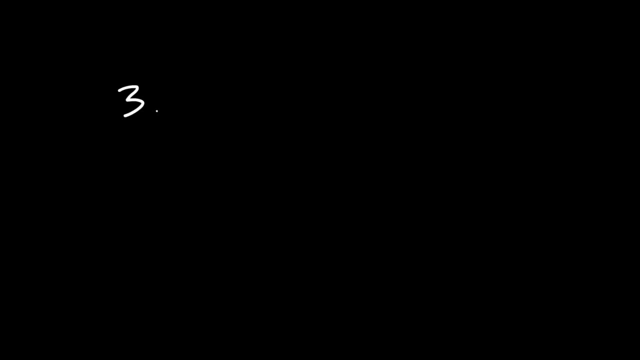 Now let's try some examples where we have to simplify the final answer. So let's multiply 3 over 2 by 4 over 9.. Go ahead and try this: 3 times 4 is 12. And 2 times 9 is 18.. 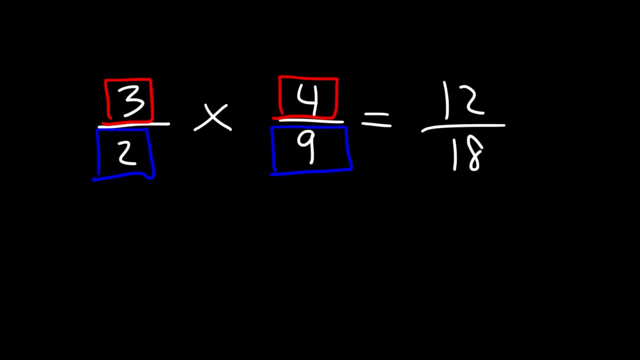 So we get 12 over 18.. How can we reduce that fraction? Now, both of these numbers are even, So we can divide 12 and 18 by 2.. 12 divided by 2 is 6.. 18 divided by 2 is 9.. 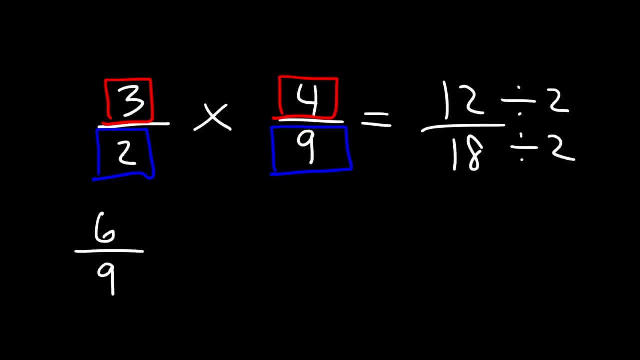 Now can we reduce this fraction, Or is that the final answer? 6 and 9 are both divisible by 3.. So we can divide both numbers by 3.. 6 divided by 3 is 2.. 9 divided by 3 is 3.. 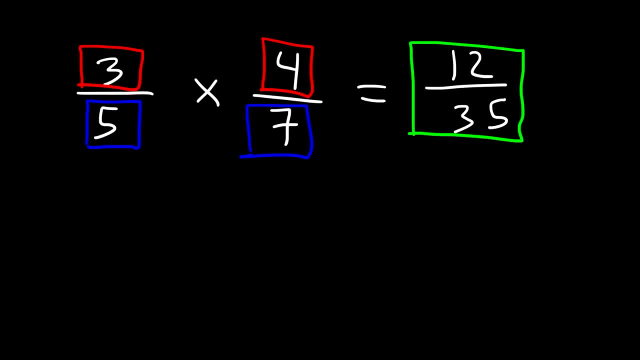 And for this example we can't simplify the fraction, So the final answer is 12 over 35.. Now let's try another example. Go ahead and multiply these two fractions: 2 over 5 times 3 over 11.. 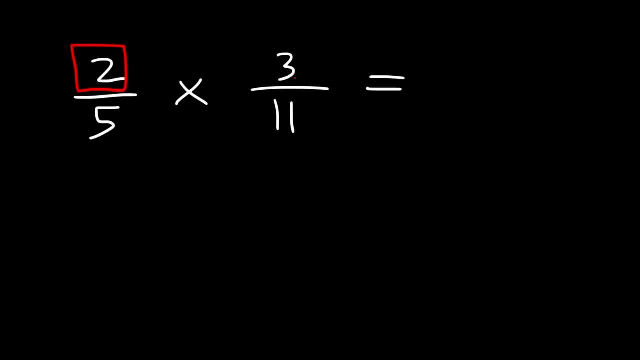 So once again, we're going to multiply across: 2 times 3 is 6.. And then we're going to multiply 5 and 11.. 5 times 11 is 55. And so this is the answer. We can't simplify this. 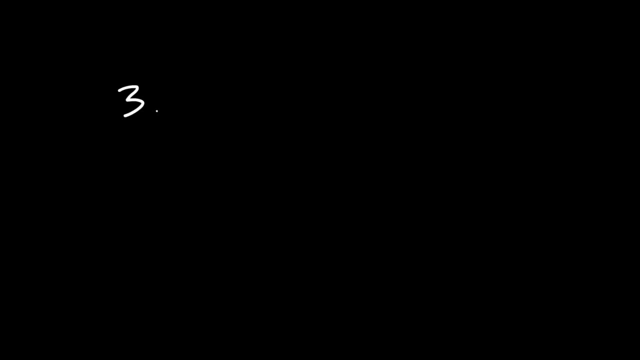 Now let's try some examples where we have to simplify the final answer. So let's multiply 3 over 2 by 4 over 9.. Go ahead and try this: 3 times 4 is 12. And 2 times 9 is 18.. 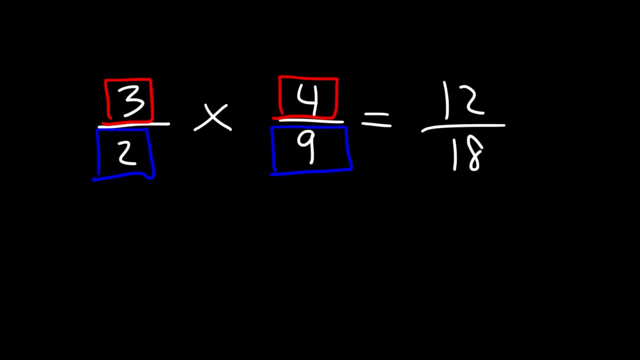 So we get 12 over 18.. How can we reduce that fraction? Now, both of these numbers are even, So we can divide 12 and 18 by 2.. 12 divided by 2 is 6.. 18 divided by 2 is 9.. 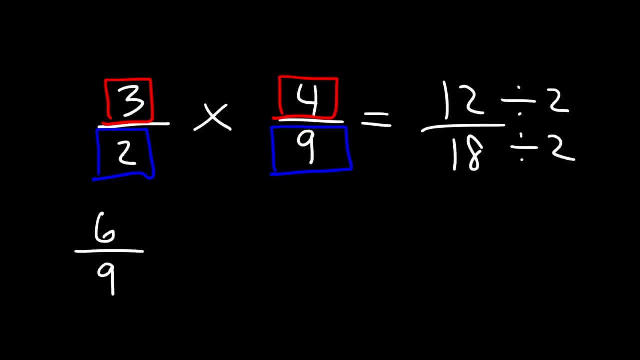 Now can we reduce this fraction, Or is that the final answer? 6 and 9 are both divisible by 3.. So we can divide both numbers by 3.. 6 divided by 3 is 2.. 9 divided by 3 is 3.. 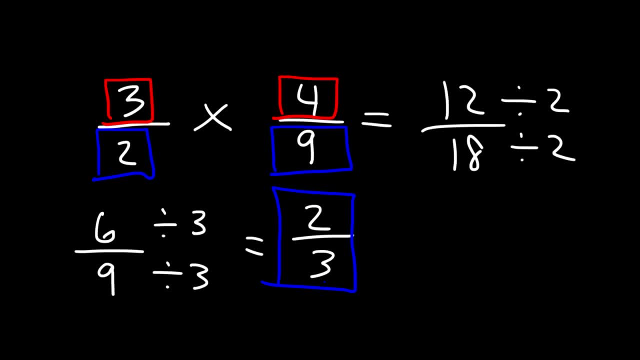 So our final answer is 2 over 3.. Now there's another way in which you can get the same answer. So once you got to let's say this part, you could do it this way. You could say: 12 is 6 times 2.. 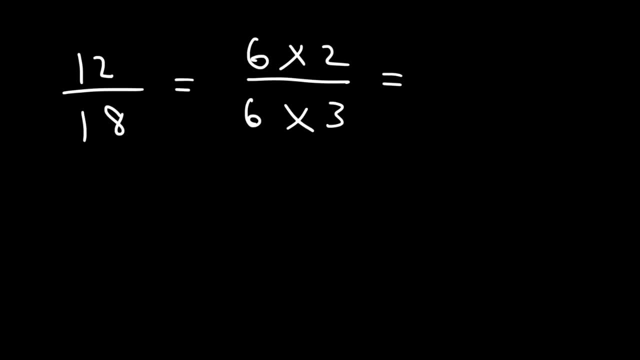 And 18 is 6 times 3.. So at this point you can cancel the 6. And this will give you the final answer of 2 over 3.. So that's another way in which you could reduce a fraction. Now let's work on another example. 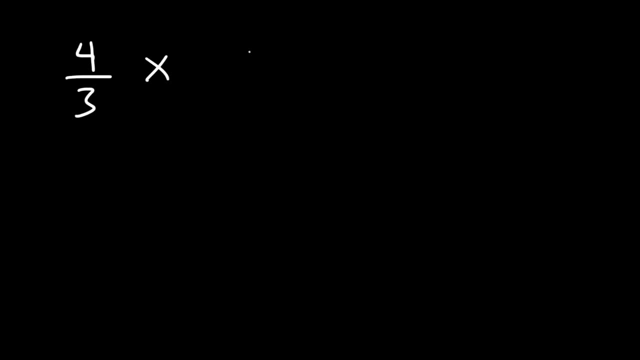 That's similar to the last one: 4 over 3 times 9 over 8.. So pause the video and work on this example. So let's multiply across: What is 4 times 9?? 4 times 9 is 36.. 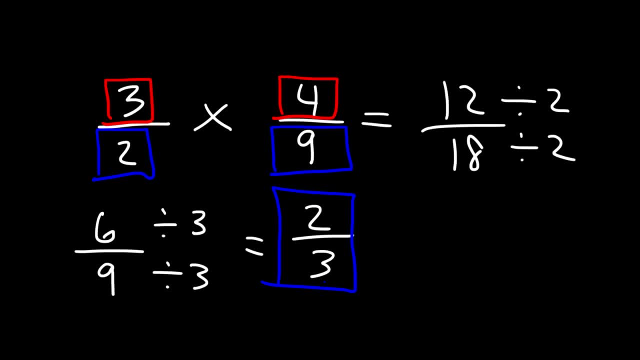 So our final answer is 2 over 3.. Now there's another way in which you can get the same answer. So once you got to let's say this part, you could do it this way. You could say: 12 is 6 times 2.. 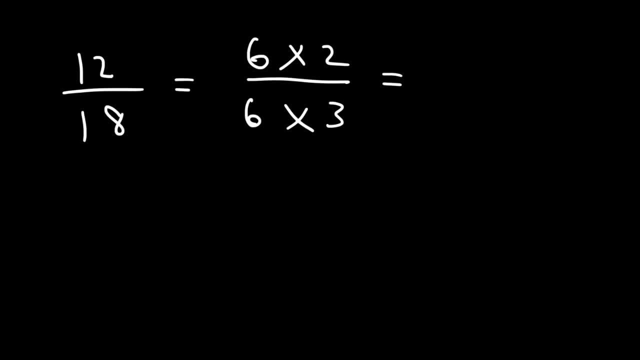 And 18 is 6 times 3.. So at this point you can cancel the 6. And this will give you the final answer of 2 over 3.. So that's another way in which you could reduce a fraction. Now let's work on another example. 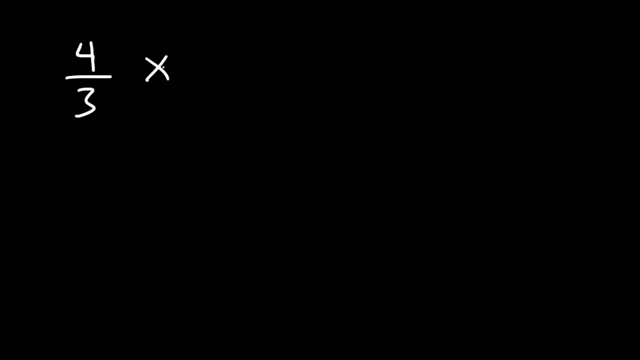 That's similar to the last one: 4 over 3 times 9 over 8.. So pause the video and work on this example. So let's multiply across: What is 4 times 9?? 4 times 9 is 36.. 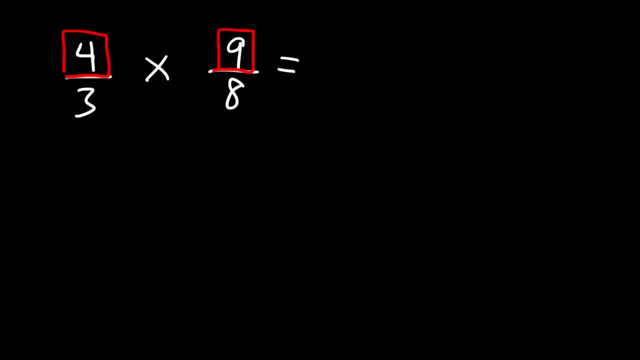 And what's 3 times 8?? 3 times 8 is going to be 24.. So how can we reduce 36 over 24?? Well, let's look at the last example. Let's look at the last example: 4 times 9 is 36.. 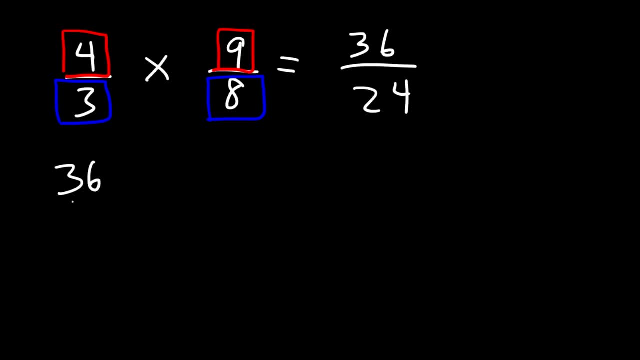 And what's 3 times 8?? 3 times 8 is going to be 24.. So how can we reduce 36 over 24? 24 and 36 are multiples of 12.. 24 and 36 are multiples of 12.. 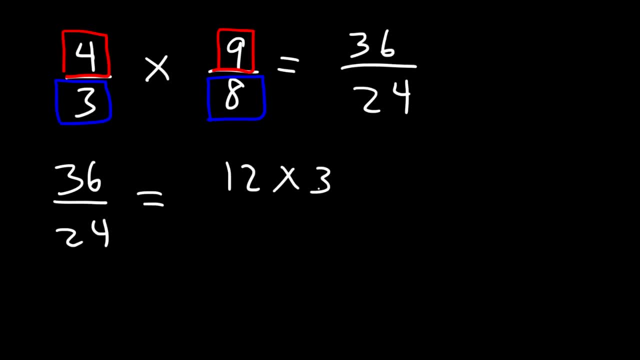 12 times 3 is 36.. 12 times 3 is 36.. And 12 times 2 is 24.. And 12 times 2 is 24.. So it really helps to know your multiplication tables. So at this point we can cancel a 12.. 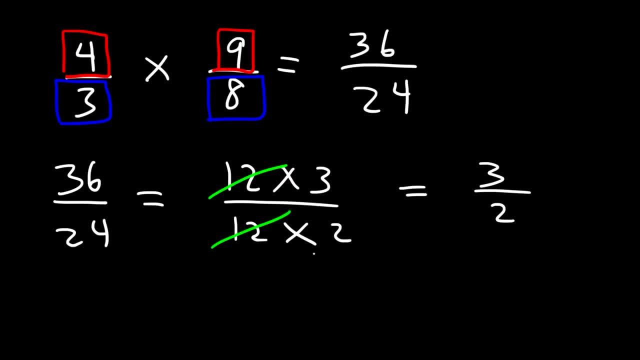 So at this point, we can cancel a 12.. And so the final answer is going to be 3 over 2.. And so the final answer is going to be 3 over 2.. Now let's talk about what to do. 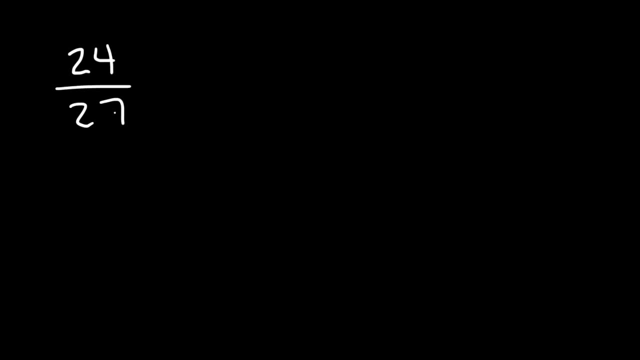 Now let's talk about what to do when multiplying two fractions that contain large numbers, that contain large numbers Such as this one. Now, what I don't recommend- Now, what I don't recommend- is multiplying across 24 times 45 is going to be a big number. 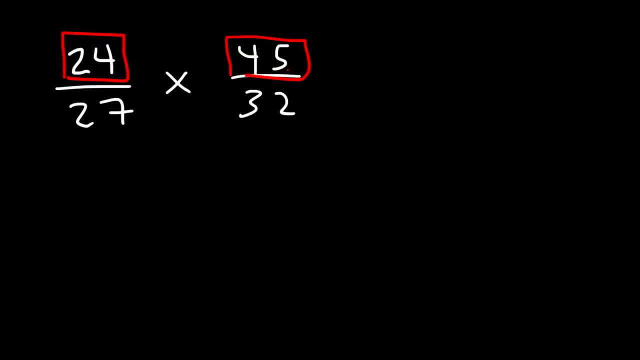 Let's see what that number is going to be If you multiply across. If you multiply across, that's going to give you 1080.. And then if you multiply 27, And then if you multiply 27, that's going to give you a large number as well. 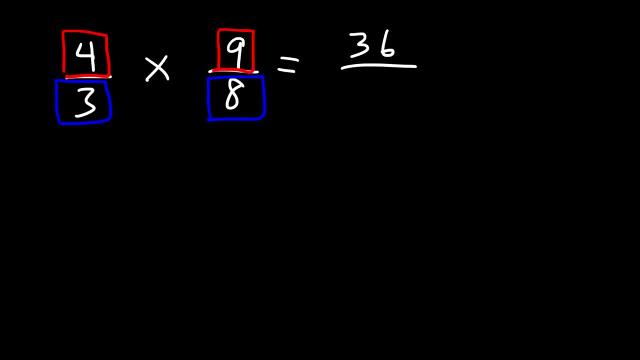 And what's 3 times 8?? 3 times 8 is going to be 24.. So how can we reduce 36 over 24?? 24 and 36 are multiples of 12.. 12 times 3 is 36.. 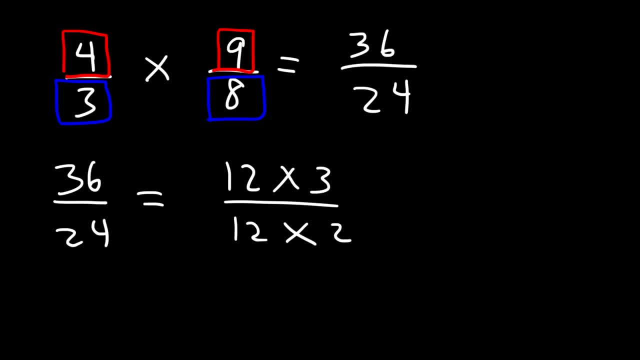 And 12 times 2 is 24.. So it really helps to know your multiplication tables. So at this point we can cancel a 12.. And so the final answer is going to be 3 over 2.. Now let's talk about what to do when multiplying two fractions. 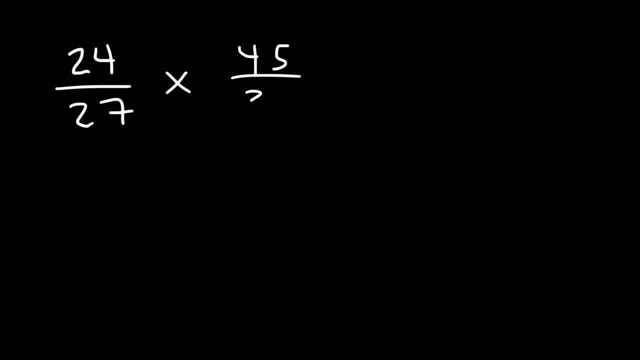 that contain 2 over 2.. How to do it right? The problem with this one is that first class is going to give you a bigger number, So the answer is A. However, A dizendo about this life超 is going to give you. 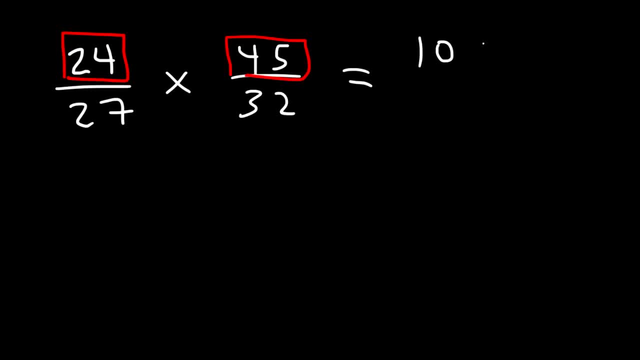 A plus A is going to give you. So, in this case, it's going to give you A plus 35, is going to give you A plus 3, is going to give you A plus 6, is going to give you a plus 4.. that's going to be 864.. So what are you going to do to reduce this fraction? That's not going to be. 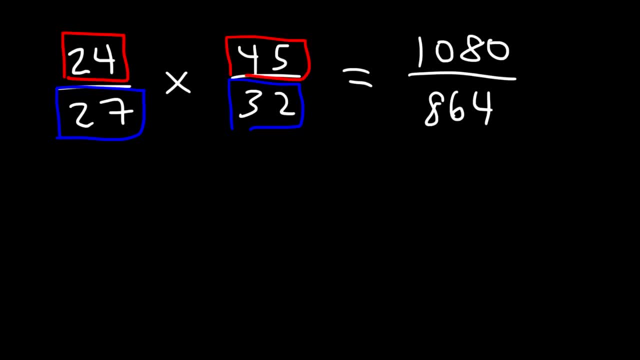 fun and it's going to take a long time. So there has to be an easier way of getting the answer for this problem, And the key is to simplify before you multiply. So, for instance, 28, we can write that as 8 times 3.. 27, we can write it as 9 times 3,, because 9 times 3 is 27.. Now 45,. you want to? 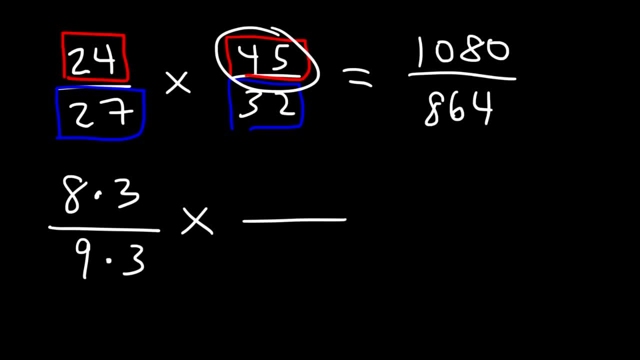 break it down into a number with a 9,, so you can cancel this 9.. It turns out that 9 times 5 is 45. And 32, we can represent it as 8 times 4.. So you want to break down these large numbers. 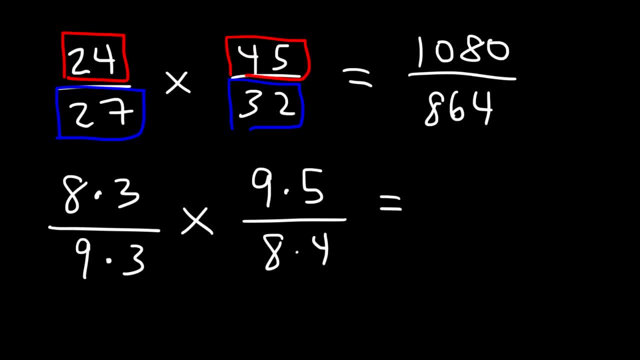 into smaller numbers in such a way that you can cancel 0.. some of those smaller numbers, So we can cancel an 8,, we can cancel a 9, and we can cancel a 3. And our final answer is just going to be 5 over 4.. 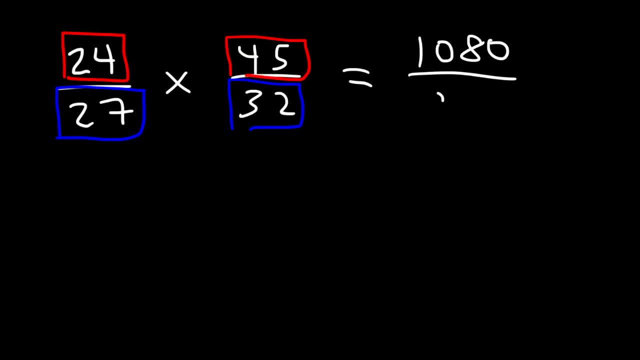 that's going to give you a large number as well. That's going to be 864.. So what are you going to do to reduce this fraction? That's not going to be fun And it's going to take a long time, So there has to be an easier way. 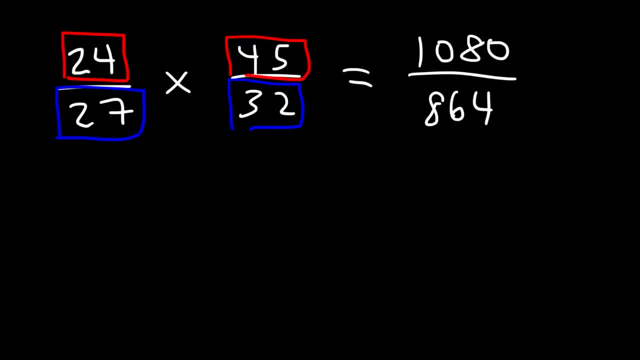 of getting the answer for this problem, And the key is to simplify before you multiply. So, for instance, 28, we can write that as 8 times 3.. 27 we can write it as 9 times 3, because 9 times 3 is 27.. 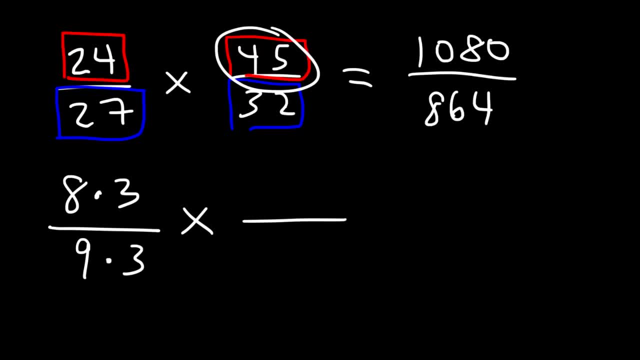 Now 45. you want to break it down into a number with a 9, so you can cancel this 9.. It turns out that 9 times 5 is 45. And 32. we can represent it as 8 times 4.. 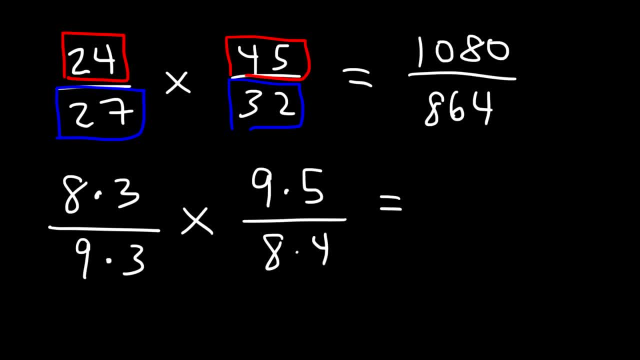 So you want to break down these large numbers into smaller numbers in such a way that you can cancel some of those smaller numbers. So we can cancel an 8., We can cancel a 9. And we can cancel a 3.. And our final answer: 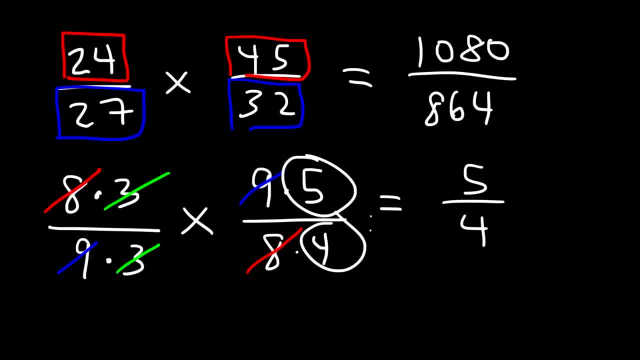 is just going to be 5 over 4.. We don't have to simplify any further than this. As you can see, this second method is a lot easier than the first. So if you have large numbers, I would avoid multiplying them to get even bigger numbers. 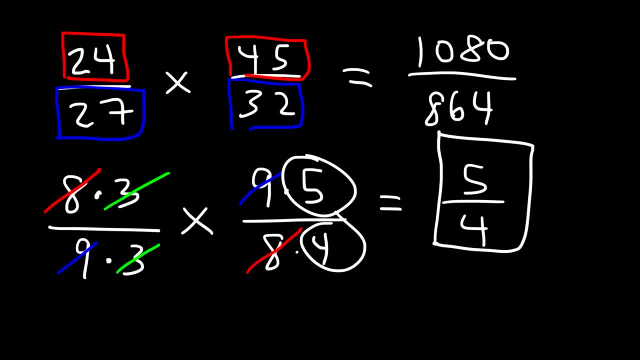 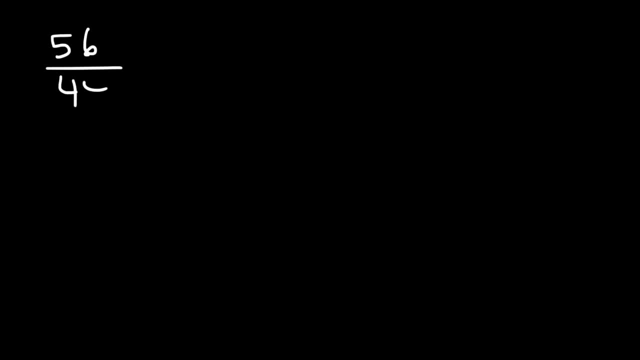 Instead, simplify before you multiply. So now it's your turn. Try this: 56 over 44 times 55 over 40. Go ahead and multiply these two fractions. So let's not multiply 56 by 55. Let's avoid that. 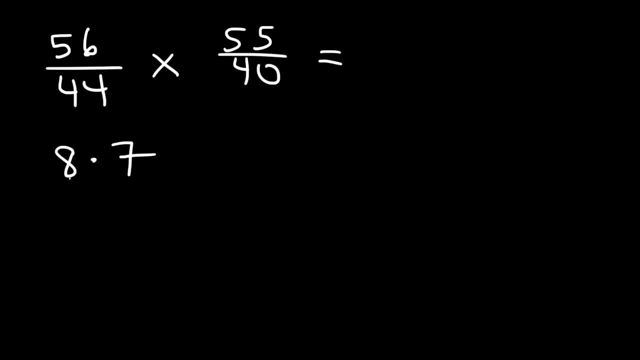 56,. we can write that as 8 times 7.. 44 is 11 times 4.. And 55 is 11 times 5.. 40 is 8 times 5.. So we can cancel an 8.. We can cancel an 11.. 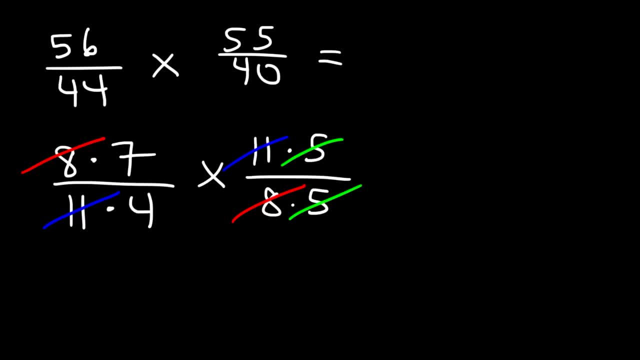 And we can cancel a 5.. So the final answer is 7 over 4.. And that's it. Now what if you get a problem that looks like this: What is 8 multiplied by 5 over 3?? How can you take? 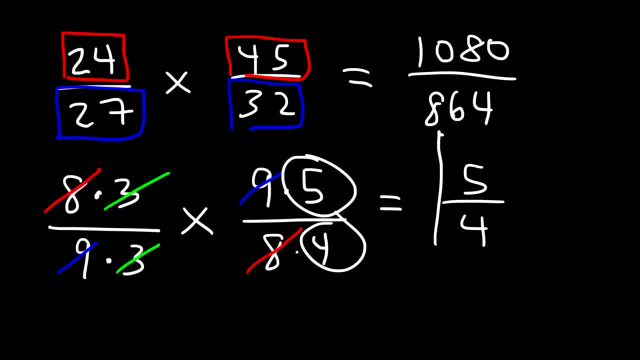 We don't have to simplify any further than this. As you can see, this second method is a lot easier than the first. So if you have large numbers, I would avoid multiplying them to get even bigger numbers Instead, simplify before you multiply. So now it's your turn. Try this: 56 over 44. 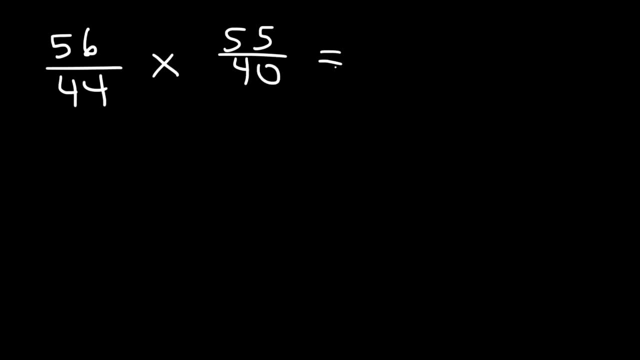 times 55 over 40.. Go ahead and multiply these two fractions. So let's not multiply 56 by 55.. Let's avoid that 56, we can write that as 8 times 7.. 44 is a lot. 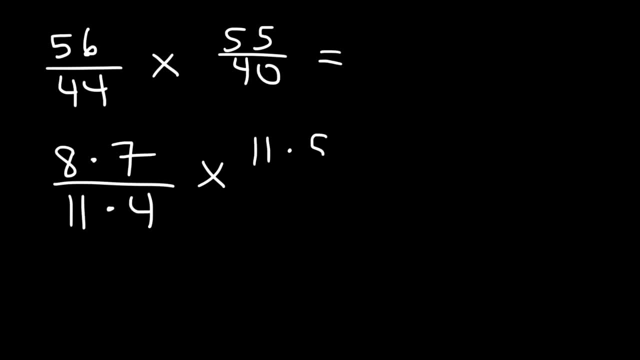 55 is 11 times 4.. And 55 is 11 times 5.. 40 is 8 times 5.. So we can cancel an 8,, we can cancel an 11, and we can cancel a 5.. So the final answer is 7 over 4.. And that's it. 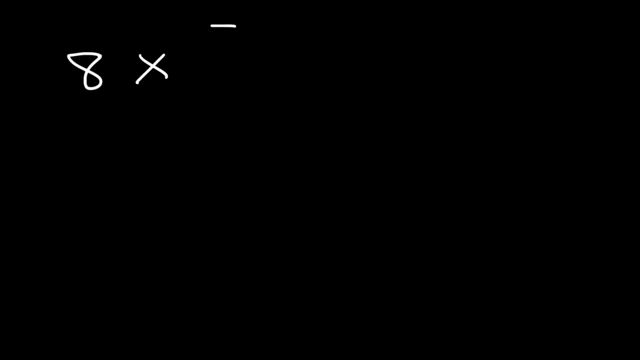 Now what if you get a problem that looks like this: What is 8 multiplied by 5 over 3?? 1 over 25 is 10 times 1,, 1 over 10, and 1 over 1.. What number is 8 is minus 3?? 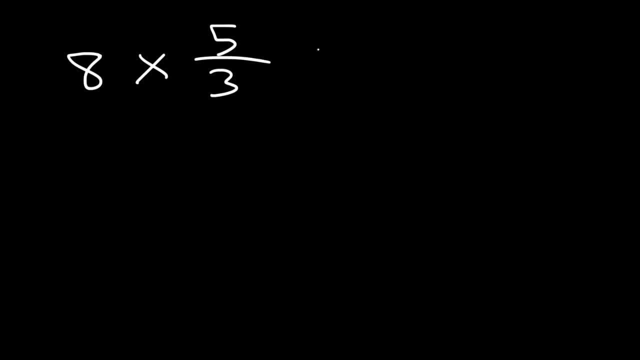 2 over орг? Or why can't you take a whole number and multiply it by a fraction? The key is to convert the whole number into a fraction. 8 is the same as 8 over 1.. In this case, 8 and 5, they are not large numbers, So we can multiply across. 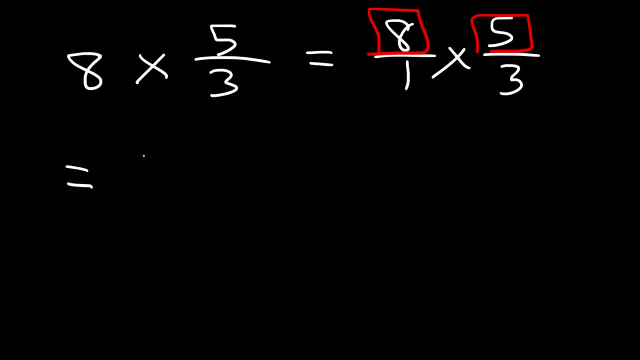 and we can't really simplify Before we multiply in this case. So 8 times 5, that's going to be 40, 10, and 13 times 9 is 10. and 3, it's going to give us 3.. So our answer is 40 over 3 as an improper fraction. 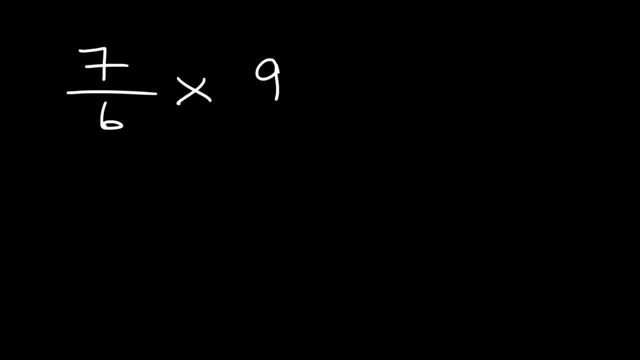 Try this one: 7 over 6 multiplied by 9.. Go ahead and work on that example. So let's rewrite 9 as 9 over 1.. Now this one we could simplify. before we multiply. if we want to 6, we can write that as 3 times 2. And 9 is 3 times 3.. So we can cancel at 3.. 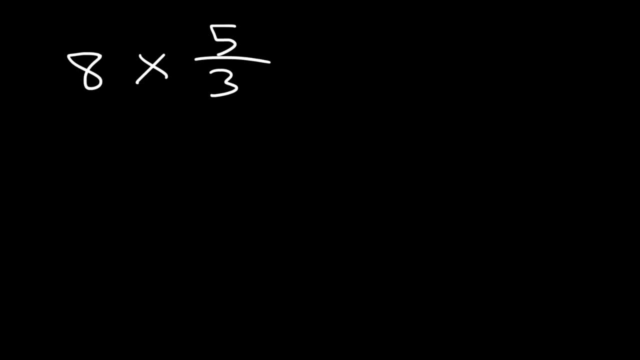 a whole number and multiply it by a fraction. The key is to convert the whole number into a fraction. 8 is the same as 8 over 1.. In this case, 8 and 5. they're not large numbers, So we can multiply across. 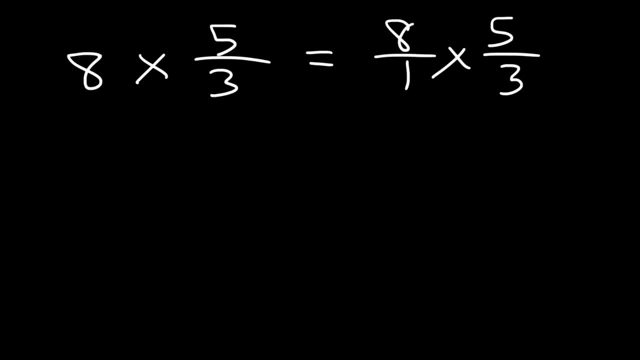 And we can't really simplify before. we multiply in this case. So 8 times 5, that's going to be 40. And then if we multiply 1 and 3, it's going to give us 3.. So our answer is 40. 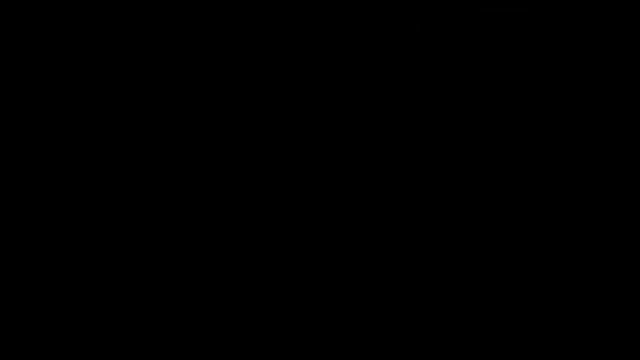 over 3 as an improper fraction. Try this one: 7 over 6 multiplied by 9.. Go ahead and work on that example. So let's rewrite 9 as 9 over 1.. Now this one we could simplify before we multiply. 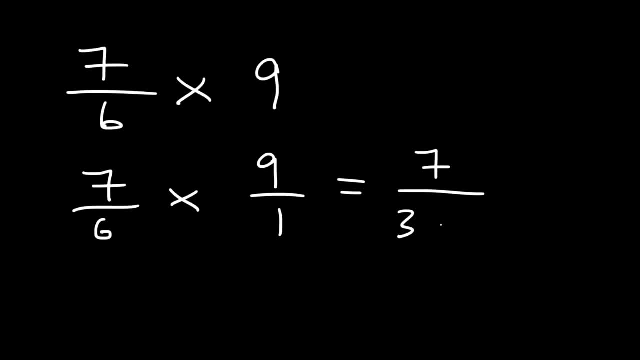 if we want to 6, we can write that as 3 times 2.. And 9 is 3 times 3.. So we can cancel a 3.. And so we're left with 7 times 3, which is 21.. 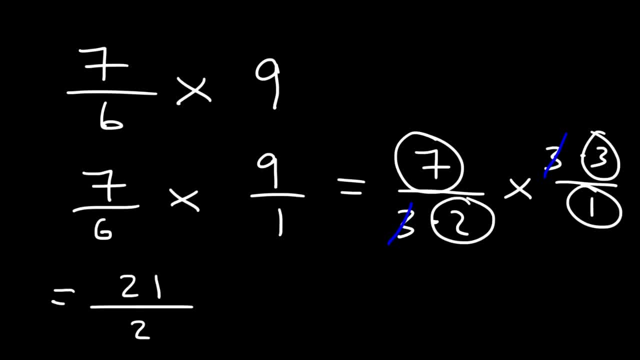 And 2 times 1, which is 2.. So the answer is 21 over 2.. By the way, if you want more videos on fractions, feel free to check out my next video on dividing fractions, Which I'm going to post a link. 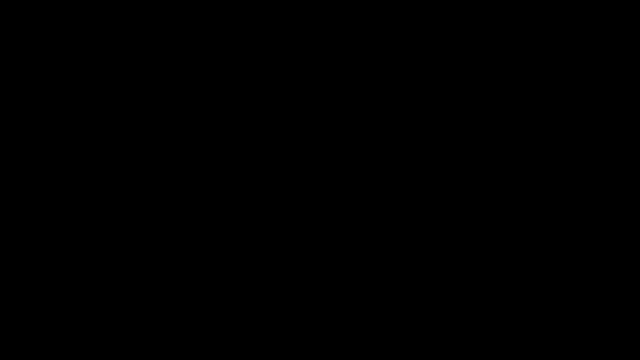 to that video in the description section of this video that you're currently watching. But now let's get back to our next problem. So let's say, if we have 12 over 28 times 18 over 30 times, 35 over 27.. 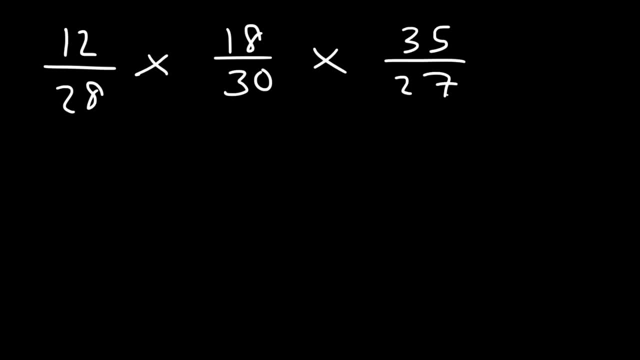 How can we multiply these three fractions? So go ahead and try this problem. 12- we can write that as 6 times 2.. 28, we could say, is 7 times 4.. 18- we can write that as 6 times 3.. 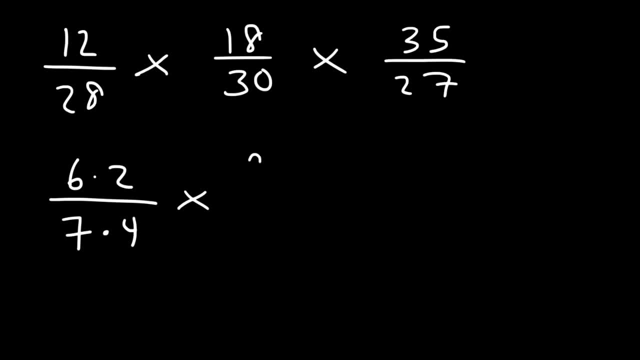 But yeah, I'm going to make that 9 times 2. Because there's a 27 and 27 is divisible by 9.. 30 is 6 times 5., 35 is 7 times 5. And 27 is. 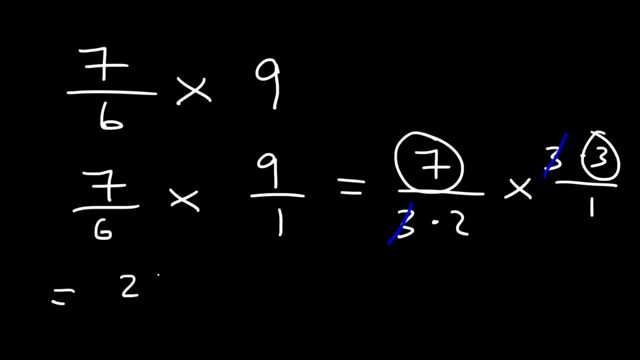 And so we're left with 7 times 3,, which is 21.. And 2 times 1,, which is 2.. So the answer is 21 over 2.. By the way, if you want more videos on fractions, feel free to check out my next video on dividing. 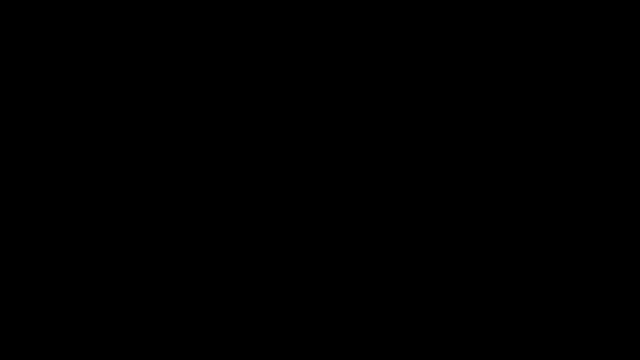 fractions, Which I'm going to post a link to that video in the description section of this video that you're currently watching. But now let's get back to our next problem. So let's say, if we have 12 over 28 times, 18 over 30 times, 35 over 27.. 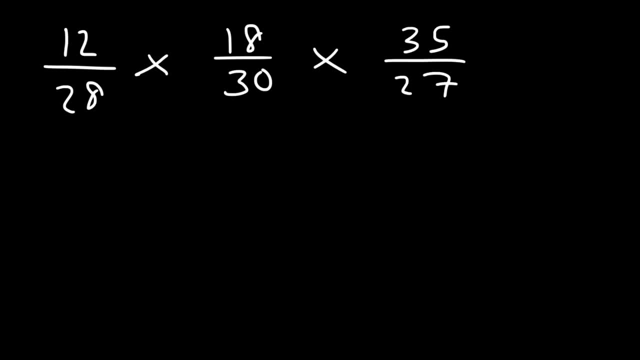 How can we multiply these three fractions? So go ahead and try this problem. 12, we can write that as 6 times 2.. 28, we could say it's 7 times 4.. 18, we can write that as 6 times 3.. 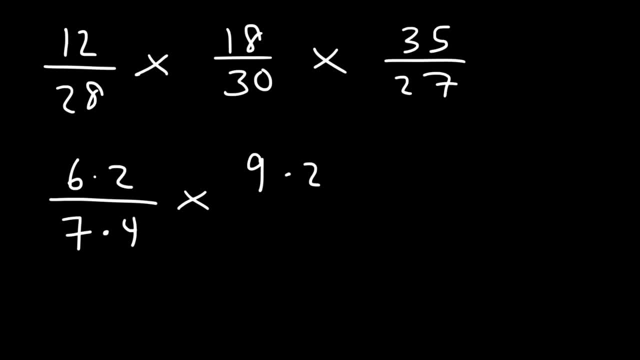 But yeah, I'm going to make that 9 times 2.. Because there's a 27 and 27 is divisible by 9.. 30 is 6 times 5., 35 is 7 times 5. And 27 is 9 times 3.. 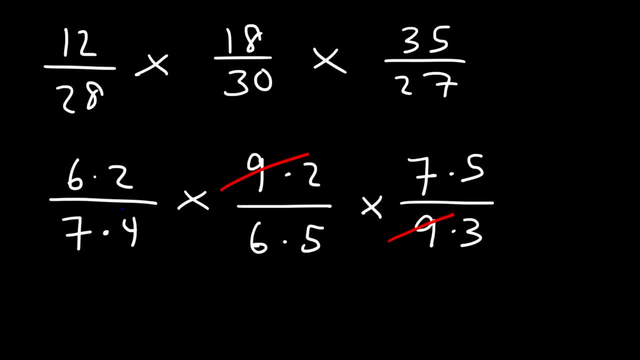 So we can cancel that. We can cancel a 9.. We can cancel a 7.. We can cancel a 5.. We can cancel a 6.. And notice that we can also cancel 4.. 2 times 2 is 4.. 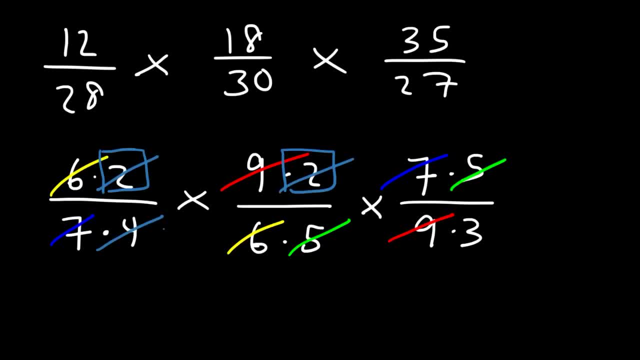 So these 2's can cancel the 4 on the bottom. So what's our final answer here? Notice that every number in the numerators of the three fractions have been cancelled. So what number should we put on top then, if there's nothing to write? 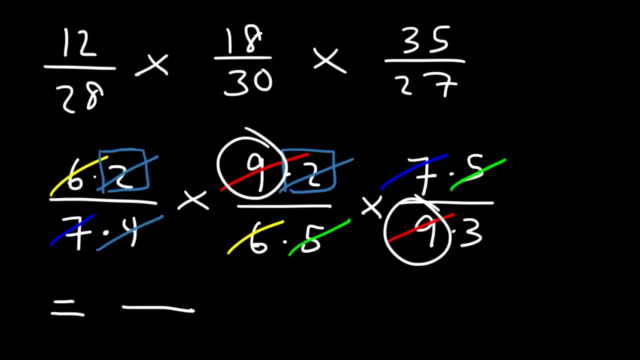 Well, if we think about this: 9 divided by 9.. The reason why that cancels is because 9 over 9 is 1.. 7 divided by 7 is 1.. So when everything cancels, the number to write is a 1.. 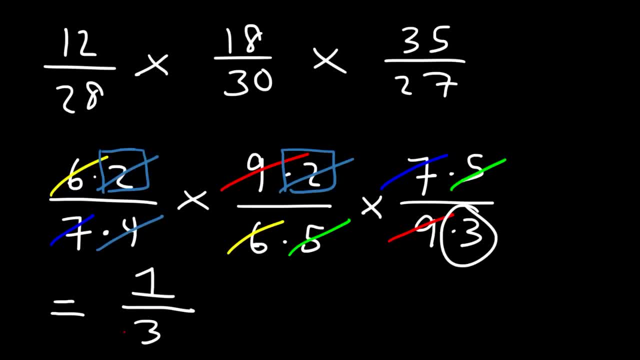 Now we do have a 3 on the bottom, So our final answer, The answer for this problem, is 1 over 3.. So this is the solution.